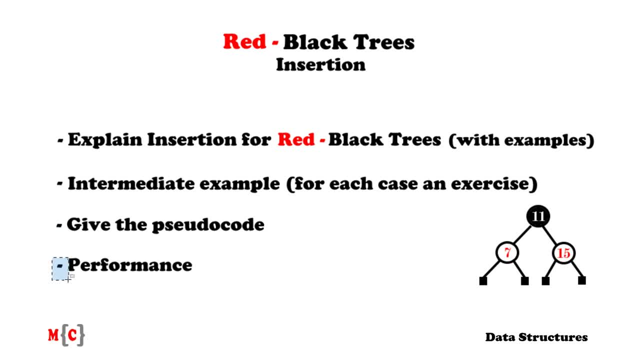 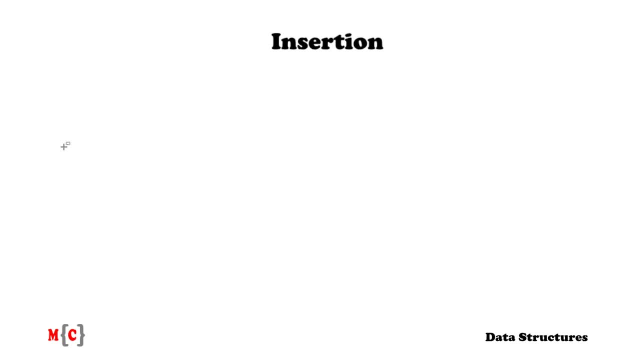 pseudo code. And finally, we will discuss the performance of the operation, But let's start with the insertion operation. Let's start with the insertion operation. Let's start with the explaining insertion for red black trees. So intuitively, if you think, in terms of insertion. 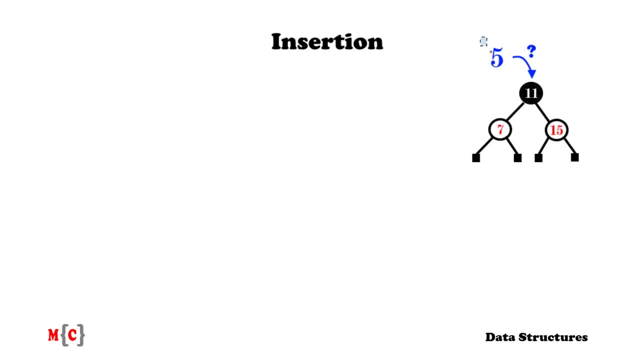 for search trees, it comes down to moving from the root of the tree to the bottom and adding a node at the end of such a path. So if we want to insert the node 5, then we would move to the left of 11, because 5 is less than 11.. We would also move to the left of 7, because 5 is also less than 7.. 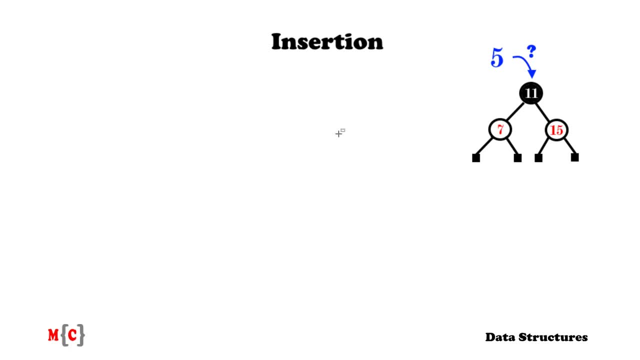 Then we would insert it here. However, this could lead to trees with all kinds of shapes, So also very unbalanced ones, And this is exactly what red black trees try to prevent. In other words, red black trees are self-balancing search trees that put some extra. 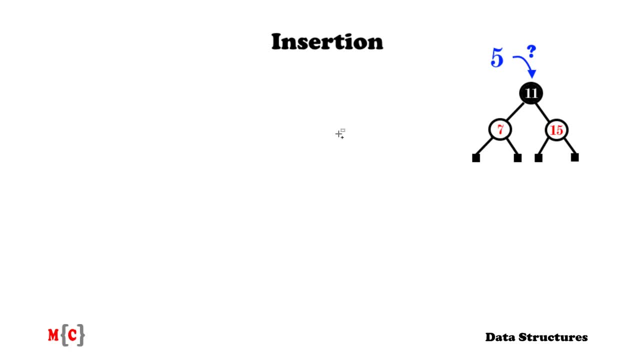 effort during insertion to keep the search tree balanced. So of course then we have this task. We have to insert node x into red black tree t And for insertion we're actually just going to consider the following decision rule, Which says that if x is the first entry, add x to t and color. 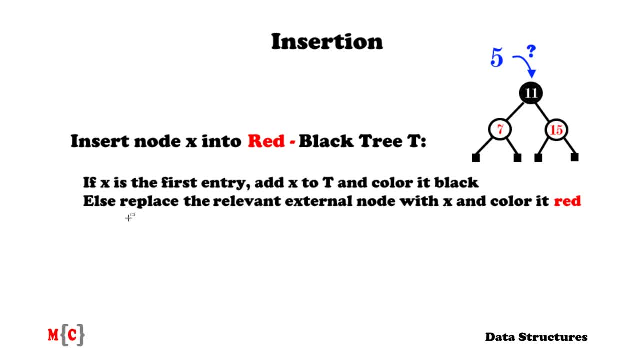 it black. So if x is the first entry, add x to t and color it black. So if x is the first entry, add x to t and color it black. And if x is not the first entry, then replace the relevant external node with x and color it red. 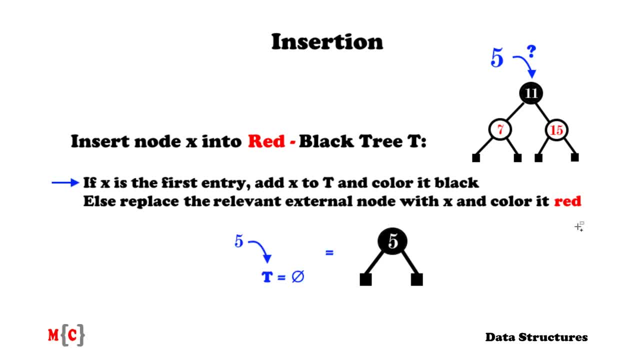 Let's see what actually happens using this decision rule. Well, in the first case, if x is the first entry of the red black tree, t, Then t would initially be an empty set. It wouldn't contain any nodes initially, And we would like to add 5 to it. Then we have the first case, So we just 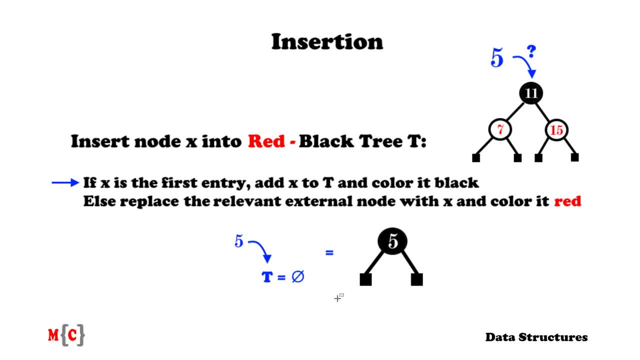 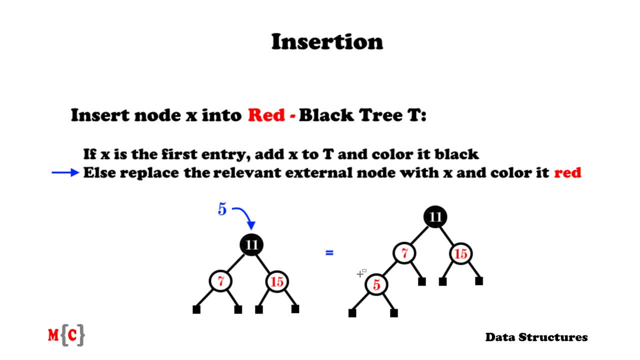 add x to t and color it black. Let's now consider the else case, using this red black tree. So we again want to insert 5, which will end up with a left of 7.. So here we replace the relevant external node with x and color it red. So now, if you think about it, Are you happy with this? 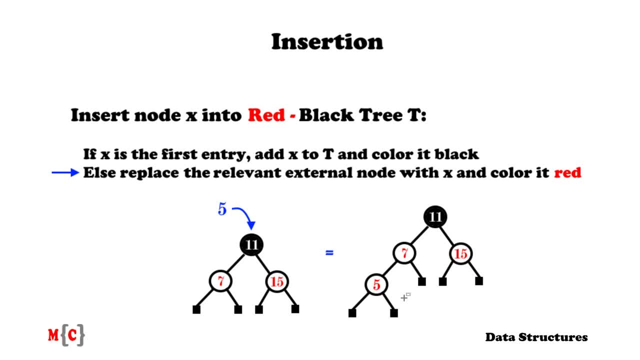 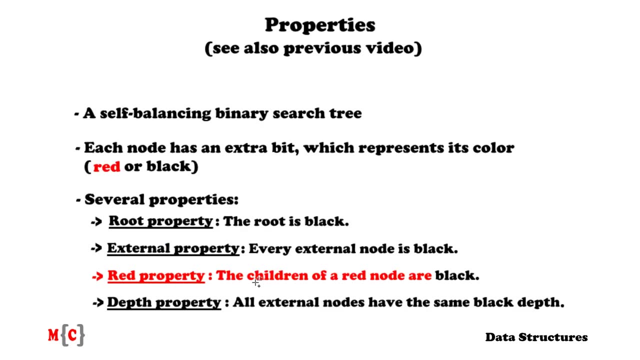 decision rule. In other words, does it still satisfy all properties of a red black tree? Well, the answer is no, But almost, Because it respects all properties except for the red property. So in the previous video, I've enumerated the properties of a red black tree, Which are the: 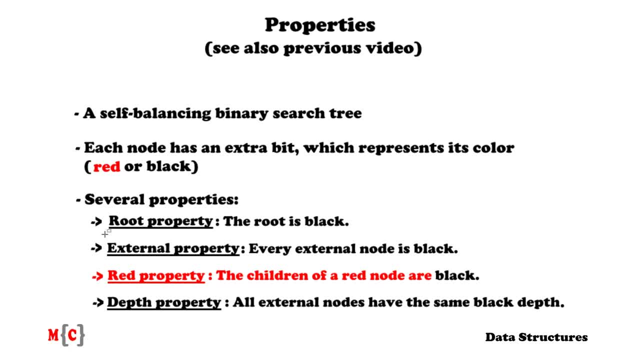 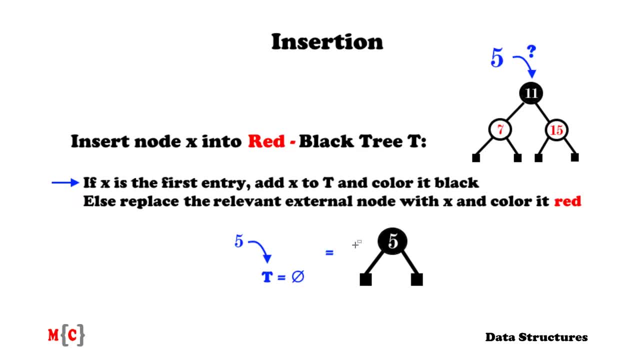 properties of the red black tree, So the root property, the external property, the red property and the depth property. Obviously, the root node is always black, Because if t was initially empty, we would add a black node, We would have a black root. We haven't changed anything about the. 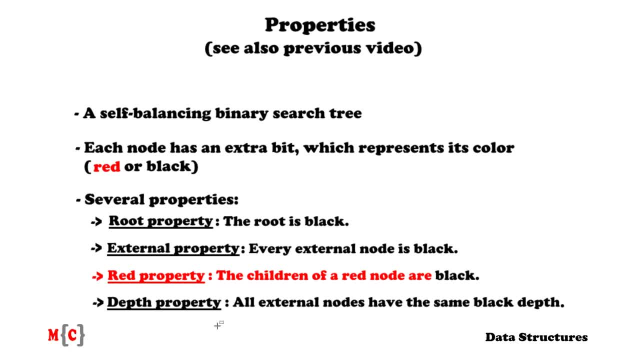 external property. Every external node is still black And the depth property doesn't change, Because we're only inserting a black node into a red black tree if it was initially empty, Which means that every path along the red black tree still has the same value, And that's why we're 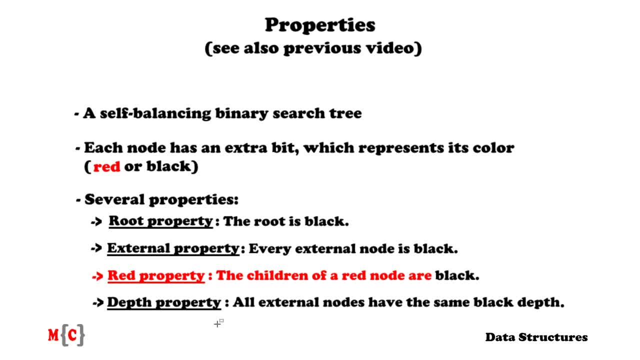 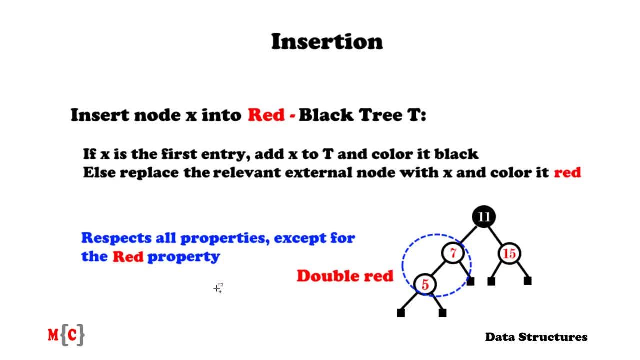 using the same black depth, But it has the same number of proper black ancestors. As I said, the red property is violated Because we're always inserting red nodes if x is not the first entry, Which means that cases like these could occur. This situation is also referred to as a double. 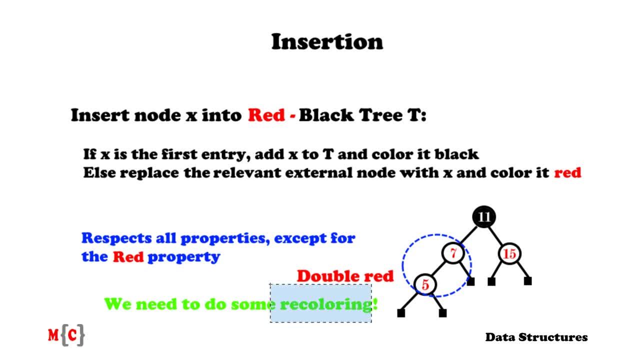 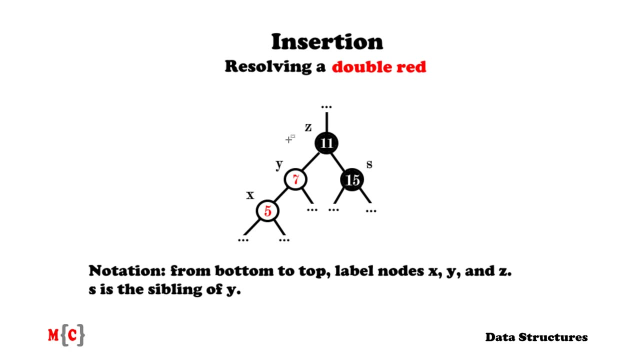 red. In other words, here we have to do some recoloring in order to resolve this. Now, taking into account this tree and the situation, Let's, for convenience, first introduce some notation. So, from the bottom to the top, we have a first label on the nodes to be x, y and z, And s will be the sibling of y. So in the previous 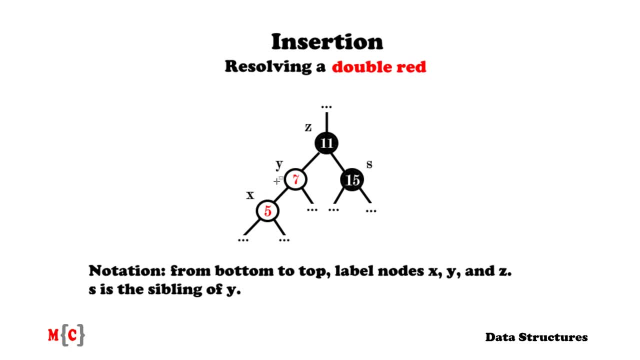 situation. we inserted x And then the parent of x is y. Therefore the grandparent of x is z And s can also be referred to be the uncle of x. Keeping this notation in mind, we will resolve a double red by performing a case distinction on the color of s, Which will help us a lot. 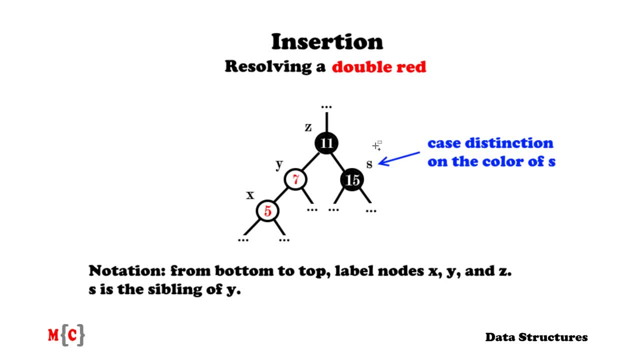 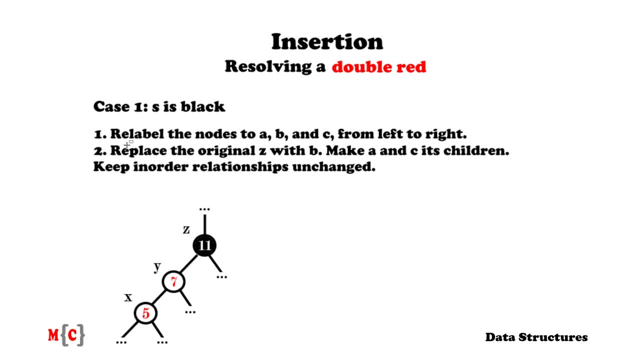 in resolving the double red. Let's first assume that s is black. Now for this case, we will resolve the double red using the following algorithm. So first we will label the nodes to be a, b and c from the left to the right, In our case below, x, y and z will become a, b and c. Then we will replace the original z with b. 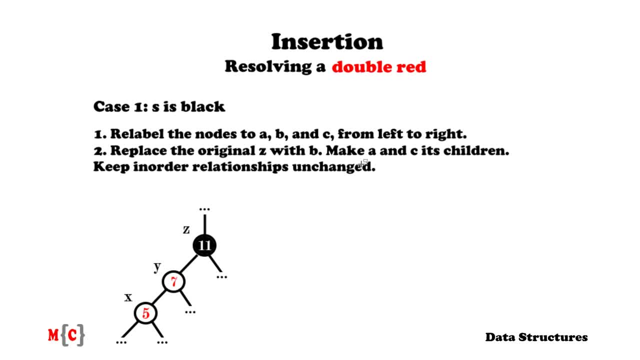 We will interchange them taking into account their color, And then we will make a and c its children, Keeping in order relationships unchanged. In this case, we will have the following: For step one, again we will have a, b and c, And now, for step two, we will interchange z and b, taking into account their 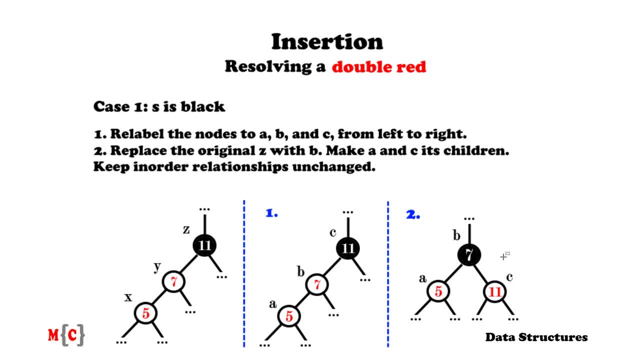 color And a and c will become their children. Now note that we will not introduce another double red because of the assumption that s is black. So in this case we will have s on the right of c, Meaning we don't introduce another double red, And this is also because we keep the in order relationship. 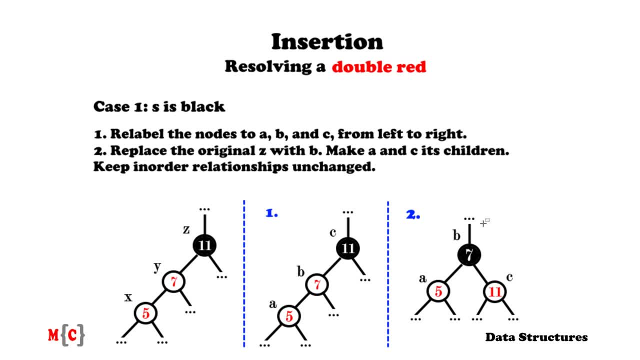 unchanged. Note that I've used three dots next to each other to indicate that the rest of the tree is independent of what happens with this subtree. taking into account the assumption, In other words, using this algorithm for this assumption, we will always respect the red black tree properties. 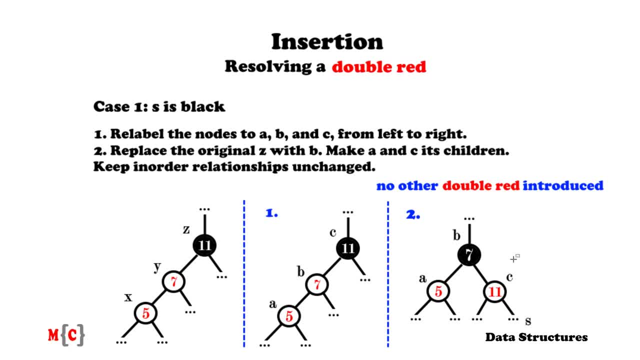 So not introducing another double red is, of course, very useful, because after this algorithm, you're basically done with resolving your double reds And you again have a nice red black tree. Now what happens if s is not black? So let's assume that s is red, like we have in this example. Well, we follow. 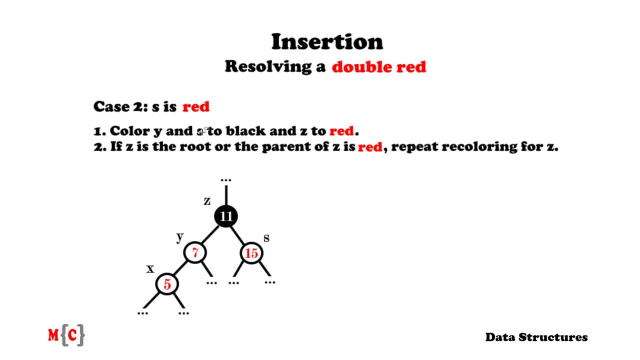 the following algorithm: First we will color y and s to be black and z to be red. So basically, this layer will become red and this layer will become black. Now, if z is a root or the parent of z is red, then we repeat recoloring for z. 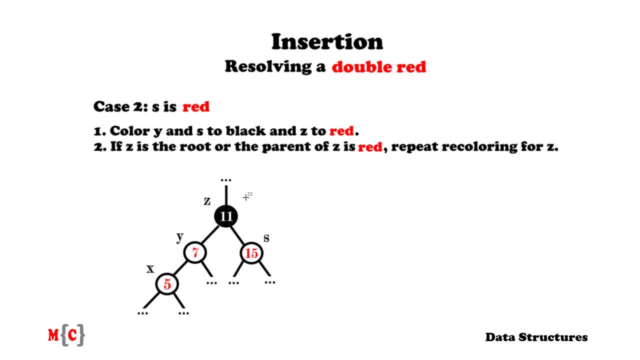 In other words, we repeat the algorithm that we have just performed. So indeed, this introduces a loop in our algorithm. So, for this example, we first recolor our nodes and then we feed it again to the algorithm, such that the newly introduced violation will be resolved by the 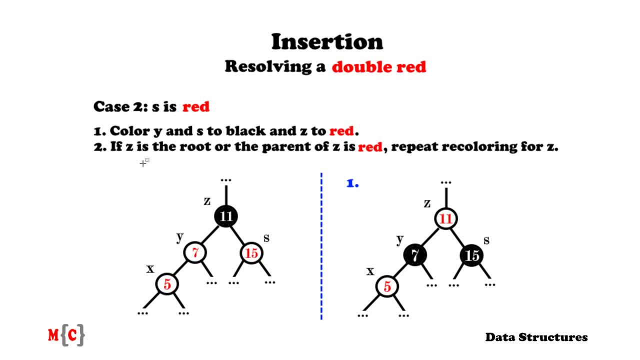 algorithm eventually, Now, if this is not the case, of course. So if z is not the root and the parent of z is not red, then we're just done and we've resolved the double red. Now. note that, because of the algorithm, the black depth is still the same, because the number of black nodes along 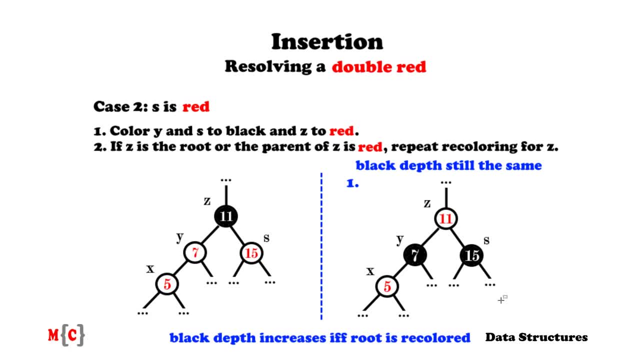 each path is, of course, yet the same. Also note that only the black depth will be increased if the root is recolored because of the iteration that occurs here. In that case we are really increasing the number of black nodes by recoloring the root to black. 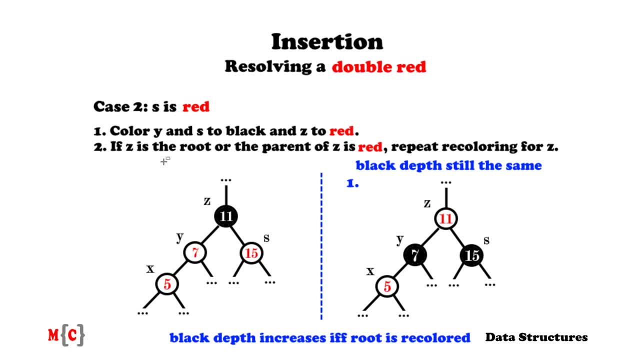 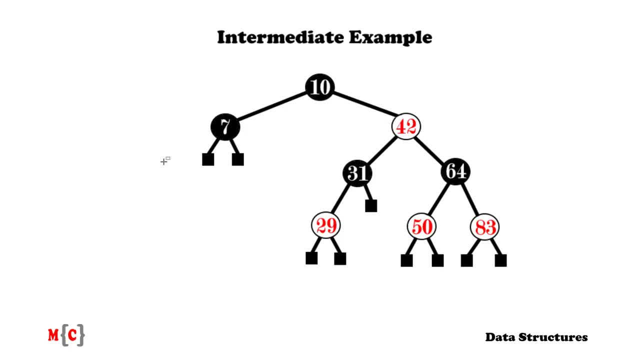 If you grasp this, you basically already understand how insertion for red black trees work. But in order to master the subject, let's do an intermediate example. I've prepared an exercise for each case, as I mentioned. Let's start with a warm-up exercise where we insert the number. 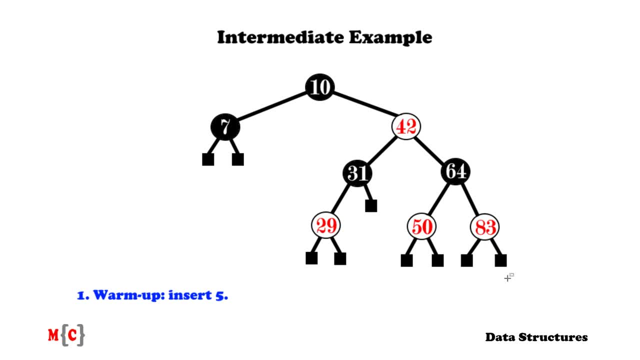 five into the following tree. Don't be scared by the size of the red black tree. I assure you that this is going to be easy. So if you would like to do this exercise on your own first, I can only encourage you to do so. Please pause the video and come back when you're done. 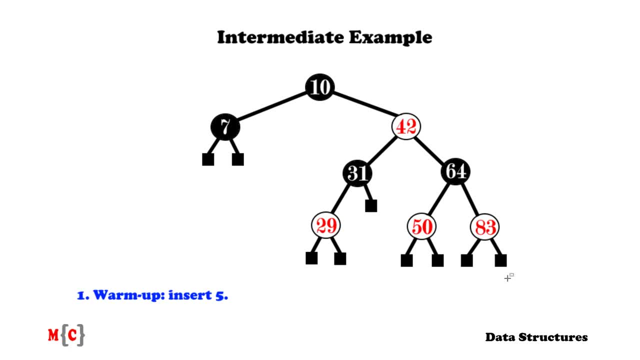 But for now I will continue with the answer to the exercise. So of course this is a rather simple exercise because we only have to insert five, as we've already done before, to the left of seven. We just replace the external node and make five red. 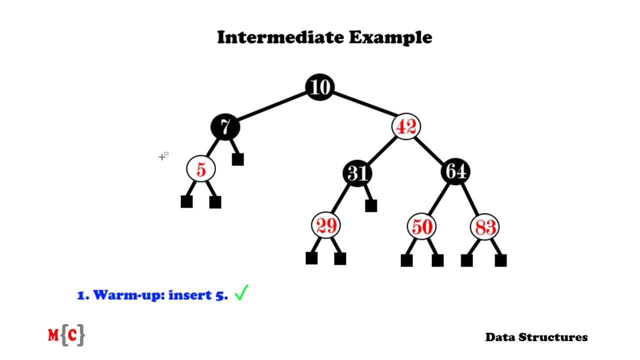 We end up with the following red black tree, where we haven't introduced the double red because seven is black. Let's now do another exercise. So here we're going to insert 23.. Again, if you want to do this exercise again first, please do so. I think it would be brave. Again. pause the video and come. 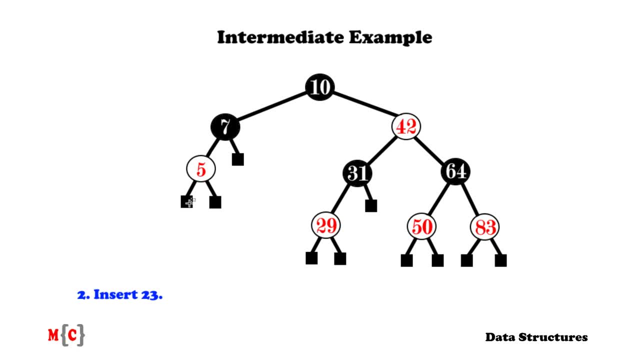 back when you're done. The answer to the exercise is to move to the left of 29.. We will replace this external node with 23, but then we will have a double red. So we need to do some recoloring And note that the sibling of y is black. So we're actually in the case where s is black. So we again. 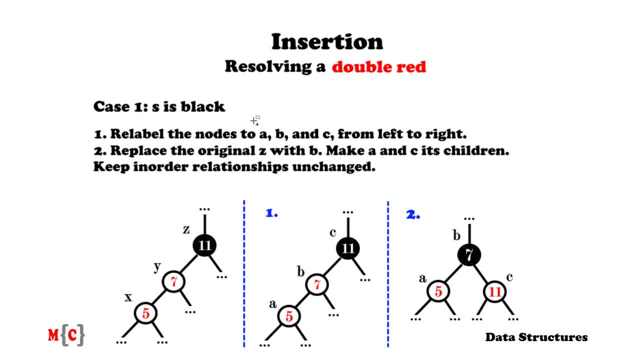 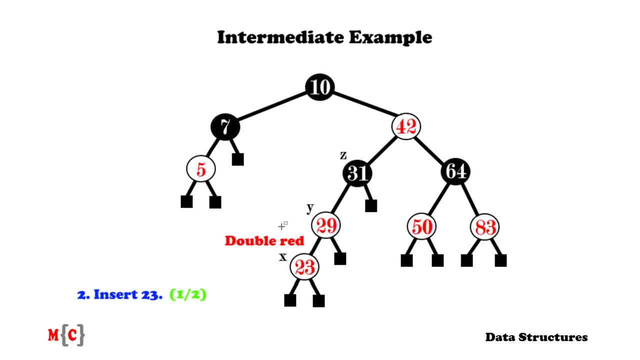 move to our nice algorithm. We label the nodes to a, b and c, from left to right, and then we replace z with b and make a and c its children. So in our example we will have x, y and z. We will label them to a, b and c, and then we 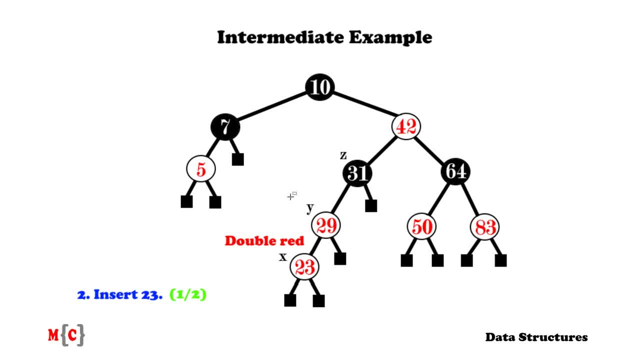 interchange z and b and make a and c its children. So we end up with the following tree. As you can see here, there won't be another double red, as is promised by this part of the algorithm. Now, I've already mentioned that we are going to do an exercise for each case, so you can. 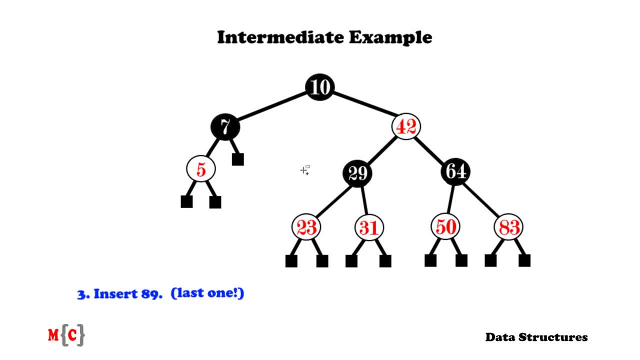 probably already guess what case this is going to be, But this is going to be the exercise. So again, if you want to do this exercise on your own first, please do so. Pause the video and come back when you're done. For now, I will continue with the answer to the exercise. For the answer, we will be. 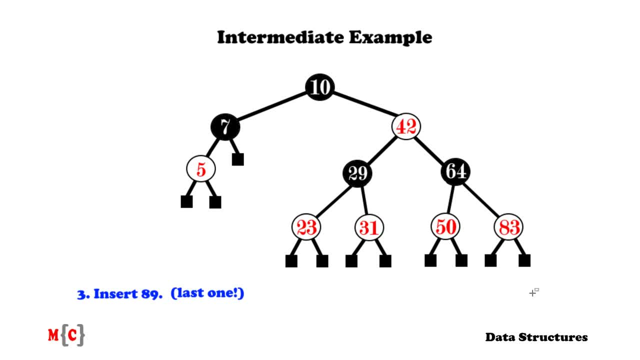 inserting 89 to the right of 83. By doing so we will of course introduce another double red For convenience. I've already indicated the labels x, y, z and s And by looking at s we see that s is red. So we have to apply our other nice algorithm where we color y and s to 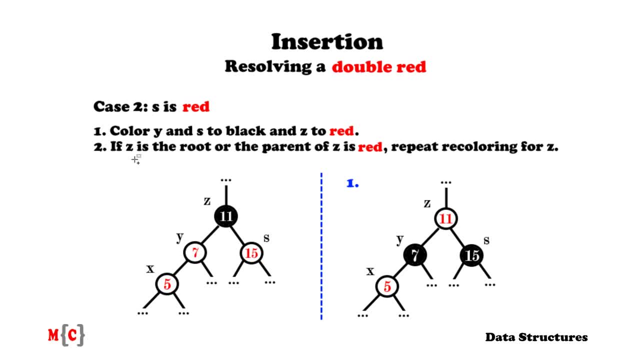 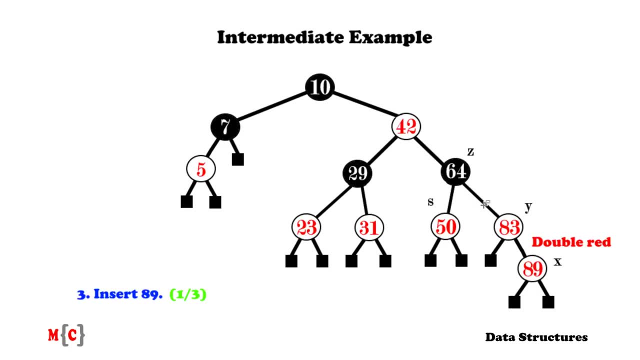 black and z to red And we will have to look at what happens with z. So if the parent of z is again red, we will have to repeat recoloring In our example. again, we recolor z to red and s and y to 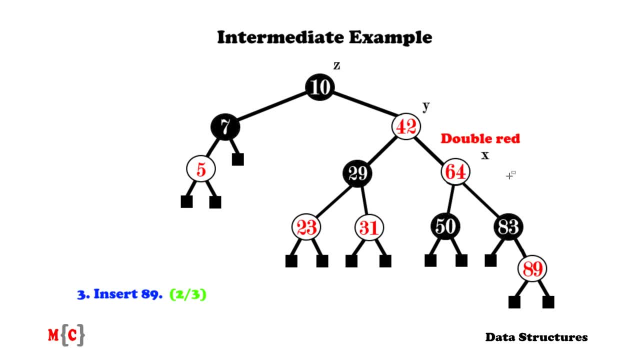 black. And then we will have the following red black tree: Here again we have another double red because we have 42 which is red. So now we've got a double red and we have 42 which is red. So now we've propagated the problem to a higher level in the tree. For convenience, I've again 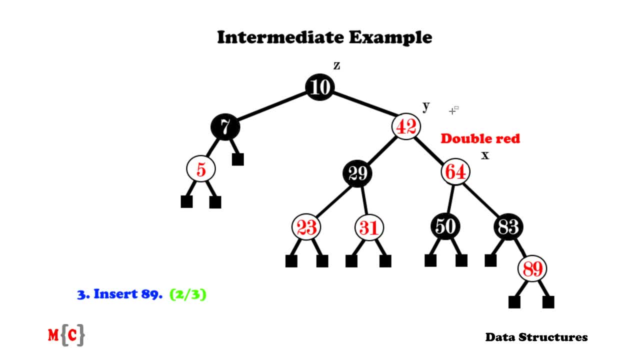 relabeled the nodes. So we have x, y and z And if we look at the sibling of y, we see that 7 is black. We can apply our algorithm when s is black. So we relabel x, y and z and interchange z and b, Make a and c its children. Therefore, we will end with the following tree, As you can see. 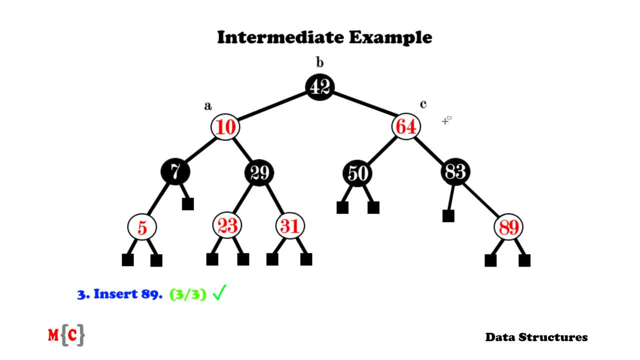 the tree seems to have changed a lot, But it's actually only because we had to keep the inorder relationship unchanged, Because we're applying this algorithm at a higher level in the tree. But, as you can see, 42 moved up and a and c became its children. 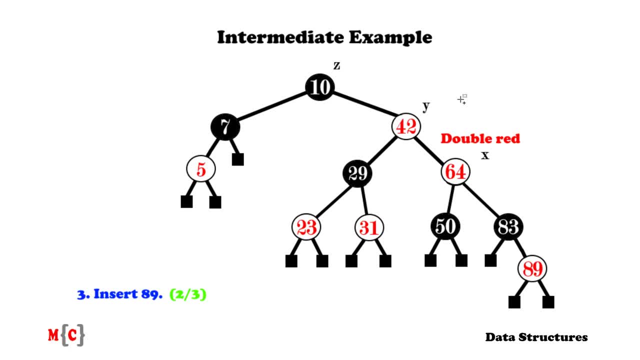 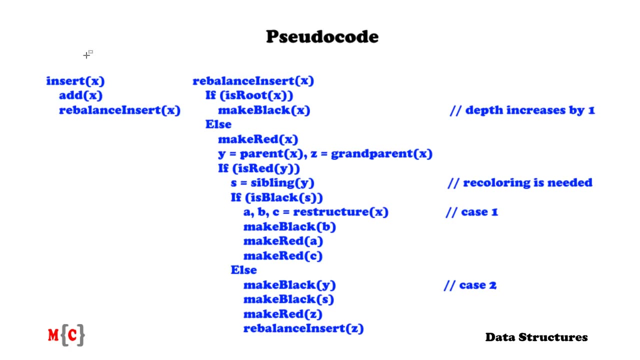 When we look at the previous step, we see that now our tree looks a lot more balanced. Okay, so by now you're basically masters of the insertion operation. So let's move on to the pseudo code of the algorithm, And I'm sure that you by now grasp this rather quickly. So we first have our insert. 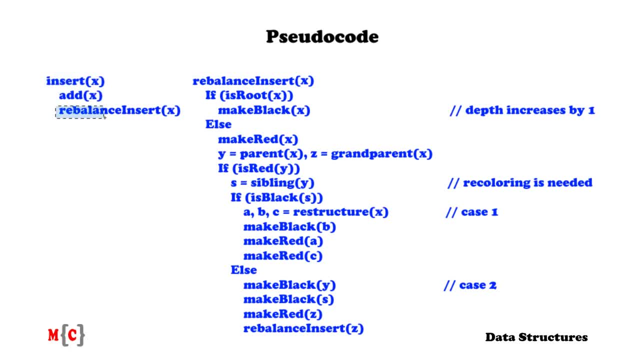 function here Which basically adds x to the subtree and then performs a rebalancing operation. During your rebalancing operation, we first check whether x is the root. If it is, then we make x black, Else we will make it red. And these lines are just based on our initial decision. 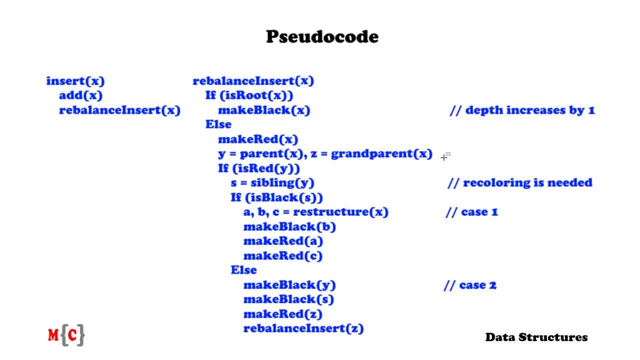 rule, And for convenience, I assign y and z to be the parent and the grandparent respectively. Now if the parent of x is red, Then we have to do some recoloring. For convenience, we assign s to be the sibling of y. Now, if s is the parent of x and z is the sibling of y, We add x to theレ and we add the Kid.